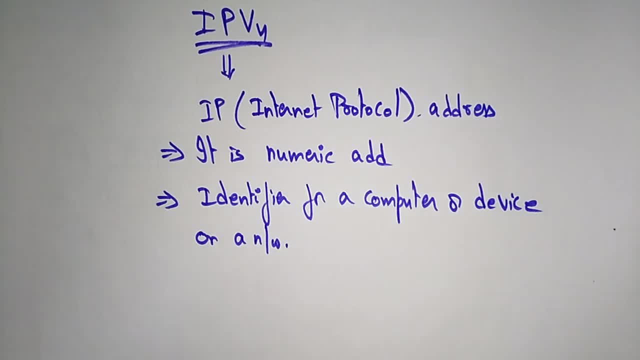 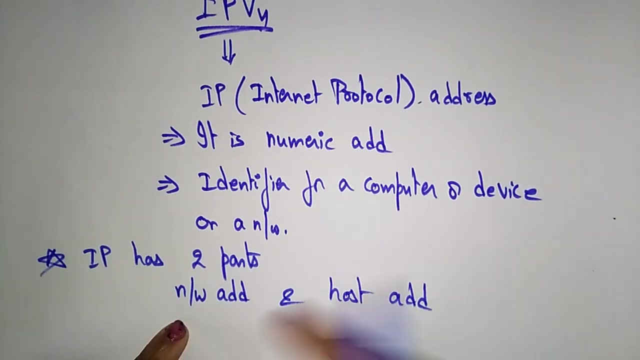 destination device. Every device has an IP address for communication purpose. So it this, the Internet Protocol, has two parts. IP has two parts. So what are the two parts? One is network address, network address, and another is the host address, Network address. So on which network you are putting the data? 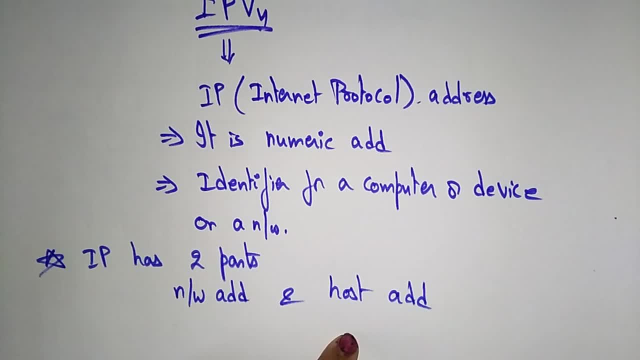 So that is a network address And the host address is nothing but the destination address, to means from where to where you are sending the data, So that IP Internet Protocol address address has two parts: One is the network address and host address, So there are two. 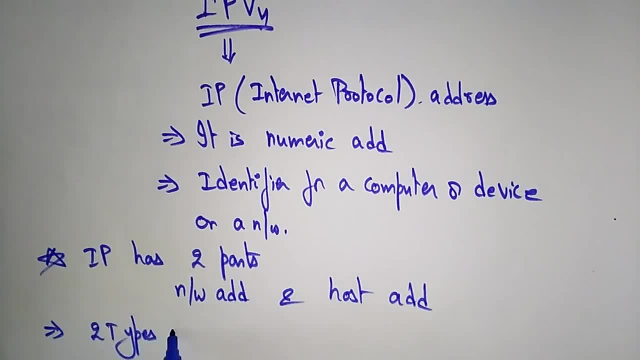 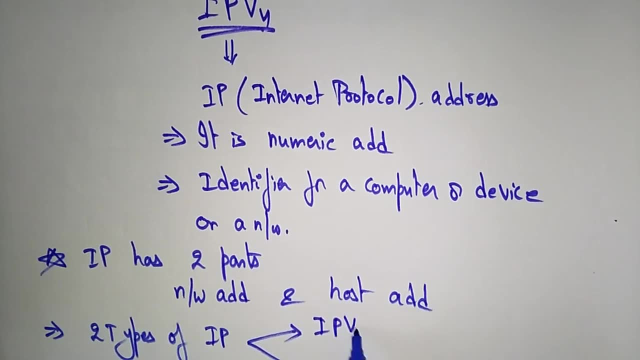 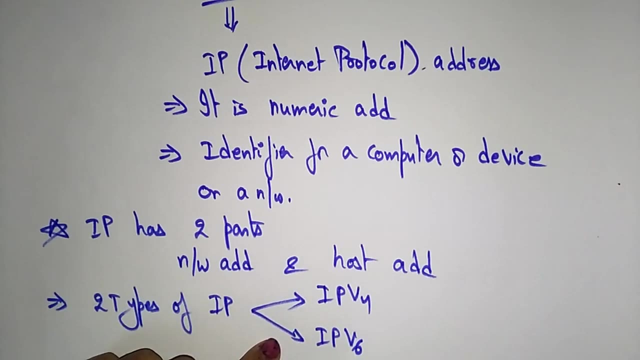 types of Internet protocols, two types of Internet protocols. So what are the two types of Internet protocols? One is the IPv4 and another is the IPv6.. That is the Internet Protocol version four, And another is the Internet Internet Protocol version six. V four is the version. 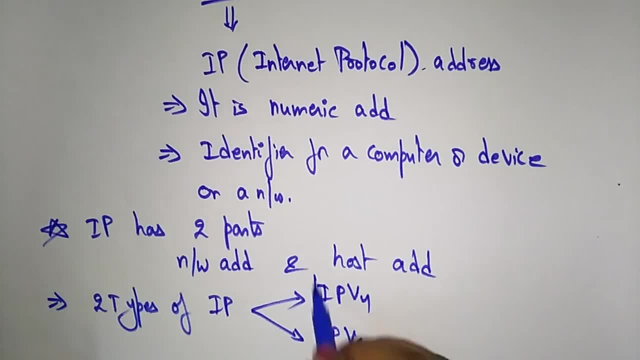 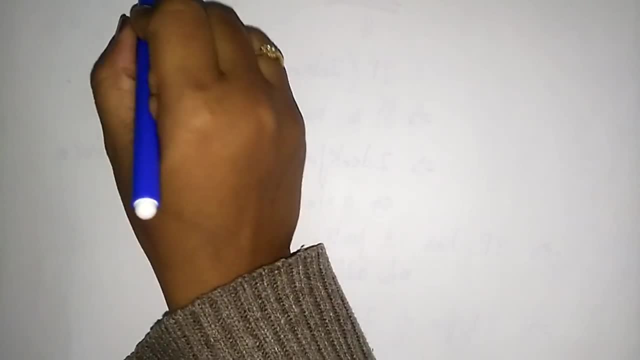 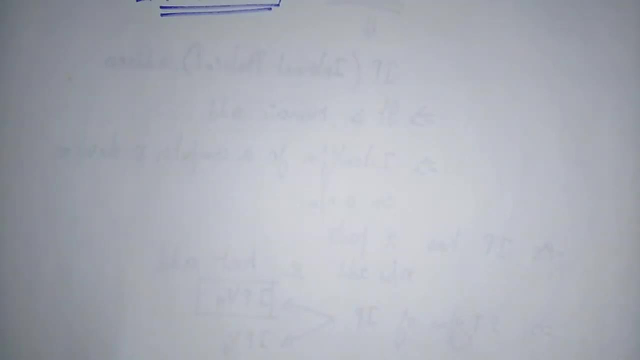 four, V, six, nothing but the version 6. let's see what is this internet protocol version 4. okay, so let me explain the internet protocol version 4. so ipv4 is the current version of ip address. so whatever we are using at present is the internet protocol version 4, so it is a 32-bit numeric address. 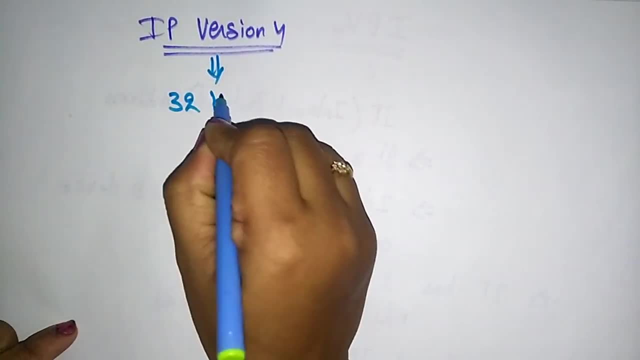 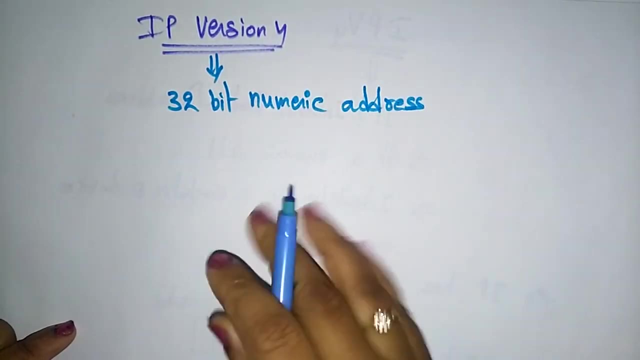 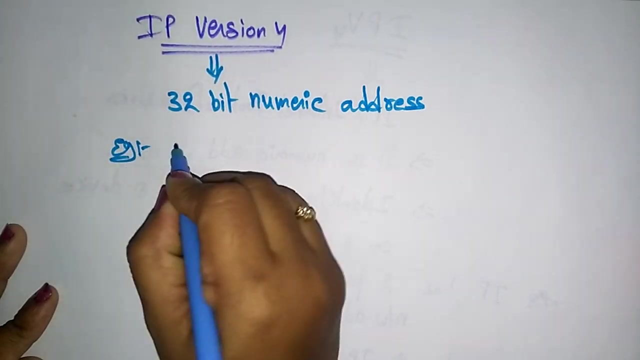 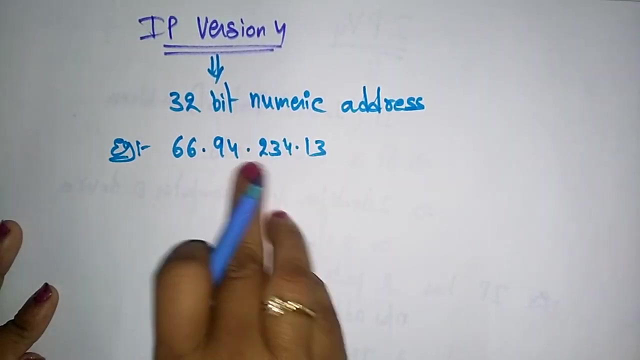 it is a 32-bit numeric, 32-bit numeric address which is written as four numbers separated by a period. so let me show you one example. it's just an example. let's let me take 66.94.234.13. so this is a period. 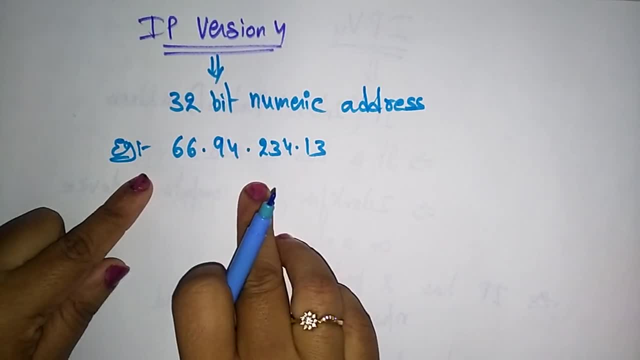 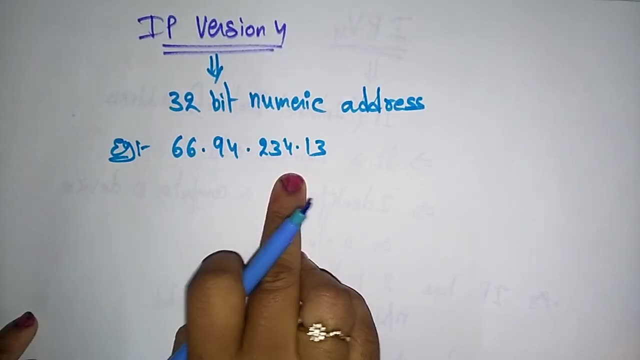 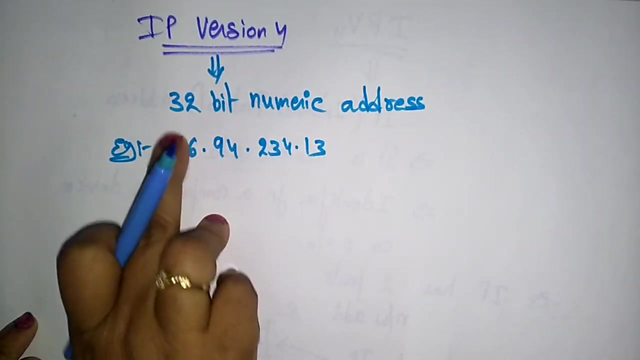 so it is a 32-bit numeric address which has written as a four numbers. so these are the four numbers separated with the dot period. so here this, each one. you call it as an octant. okay, each number with the dot period, this is one octant. 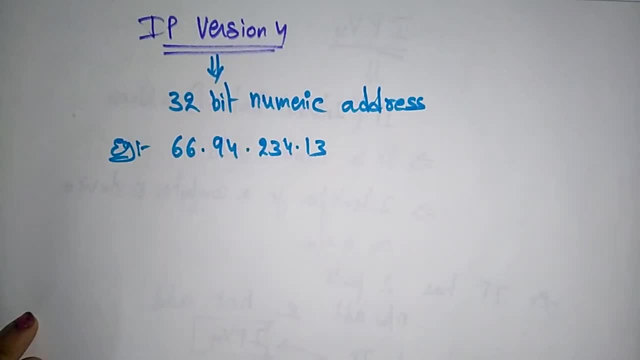 another octant octant. octant octant is number of range, so the complete range is range of octant. so, whatever you are taken, that octant range is from 0 to 255. so this range is 0 to 255. this octant range is 0 to 255, like that, whatever the octant you are taken, that range is. 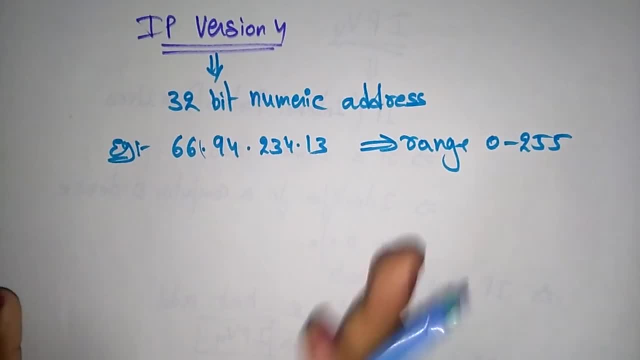 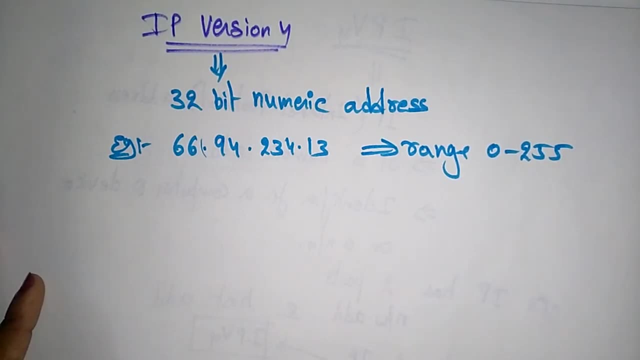 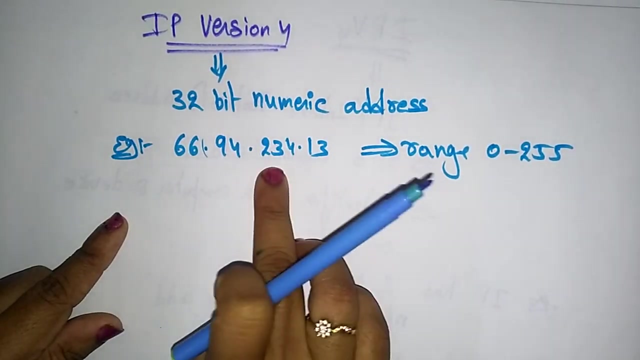 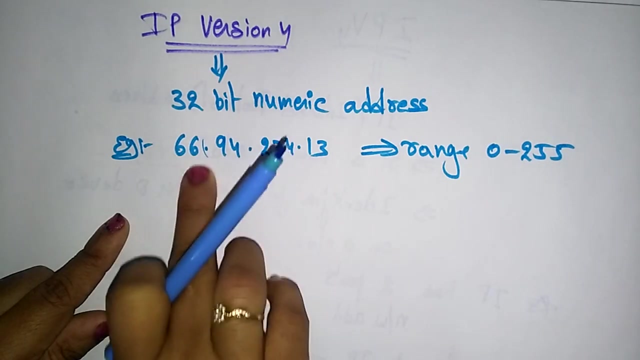 from 0 to 255. okay, so don't be confused. internet protocol version 4 is a current version of ip address. whatever we are using, it is a 32-bit numeric address. okay, that 32-bit numeric address written as a four numbers? okay, four numbers separated by a dot period. so each part you call. 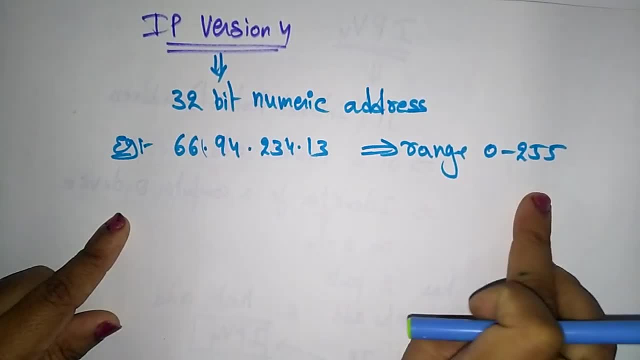 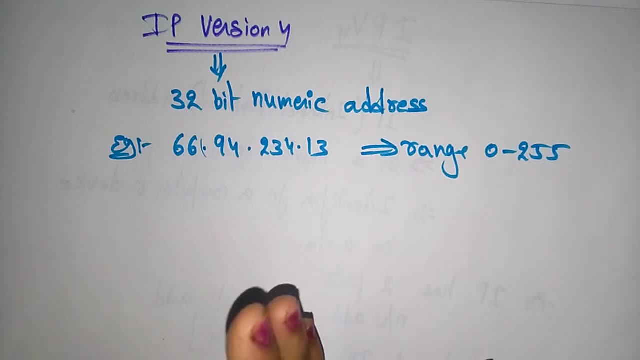 it as an octant. this octant should be in the range of 0 to 255. okay, so here, the computer and network don't read the ip address in this standard numeric format. okay, so actually, if you written like this, the computer and whatever the network that you are placing the data so it doesn't. 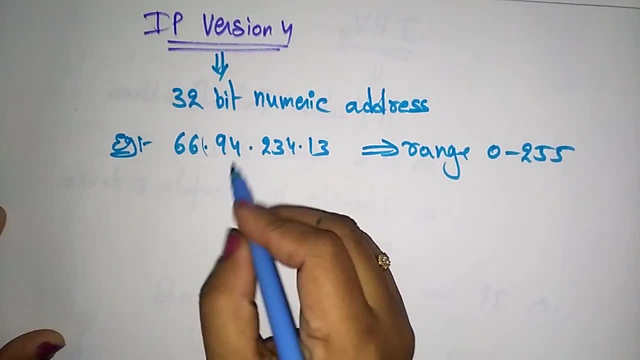 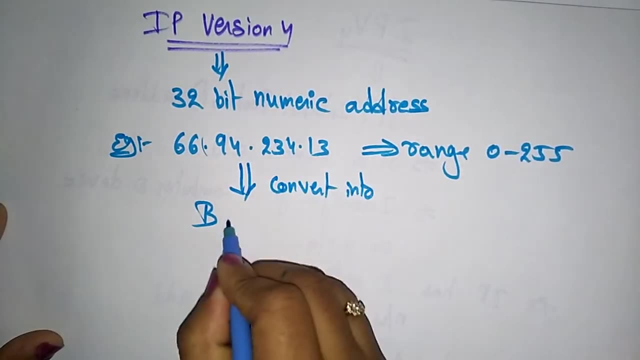 understand. so whatever the numeric address you are given, that will be converted into binary format. okay, convert into. convert into binary format. binary format mean it's nothing but numbers in the form of ones and zeros. now let's see the binary number for an ip address. so, whatever the 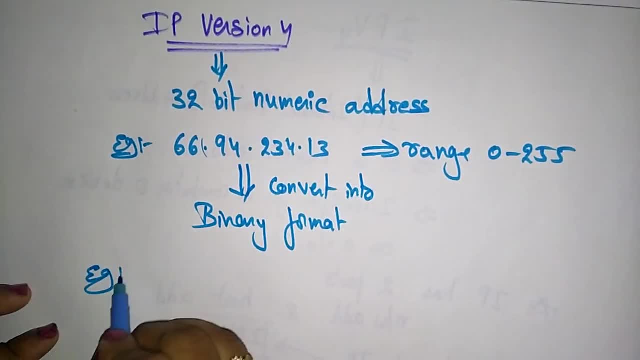 ip address, here you are given. let me take another example. so let me convert the find out, the okay, Find out binary number for an IP address which is written in: let's take 66.94.29.13.. So this is the IP address which is in the decimal form. 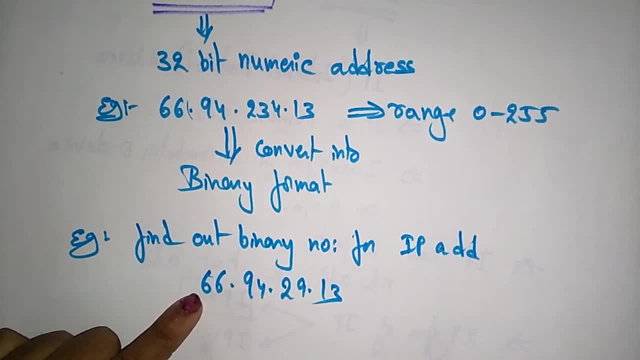 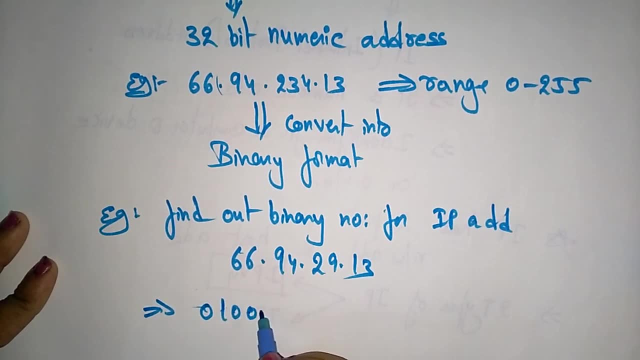 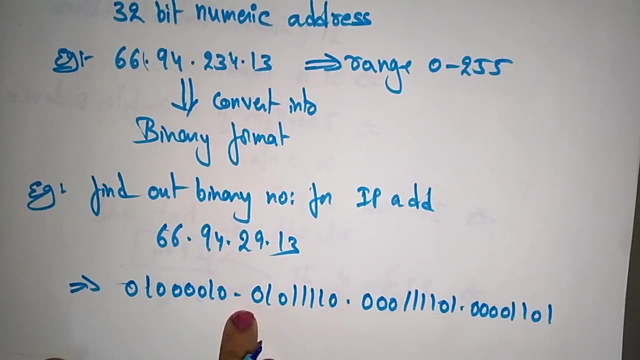 I want to convert into binary number so that the system can understand. So how you are going to convert. Actually, the answer for this you will get is the conversion is 01000010.. So this is a binary conversion for this decimal numbers. How you will get this. 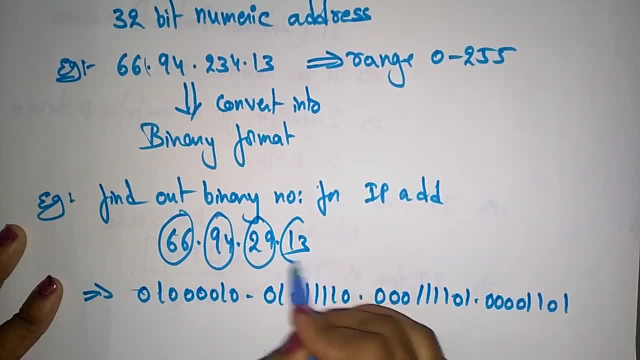 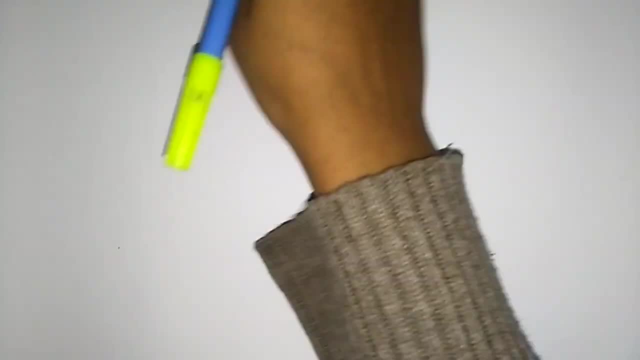 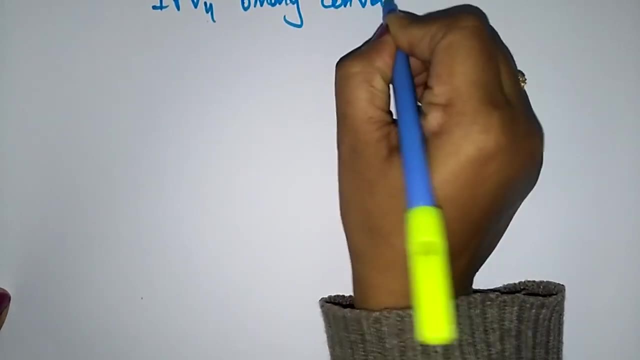 Let me see, Let me take each octant and explain how I get this number. So let me take the binary conversion: IPv4. binary conversion- IPv4- binary conversion, So actually the 8-bit octant chart, how it will look like. 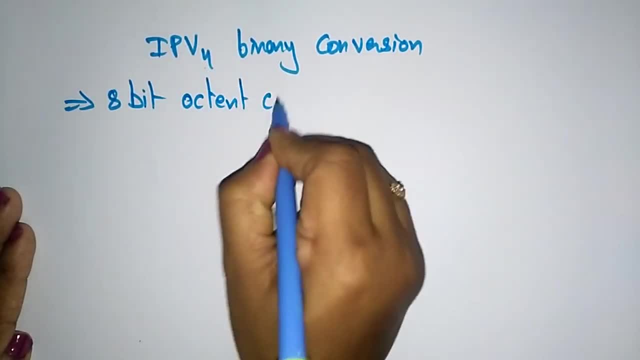 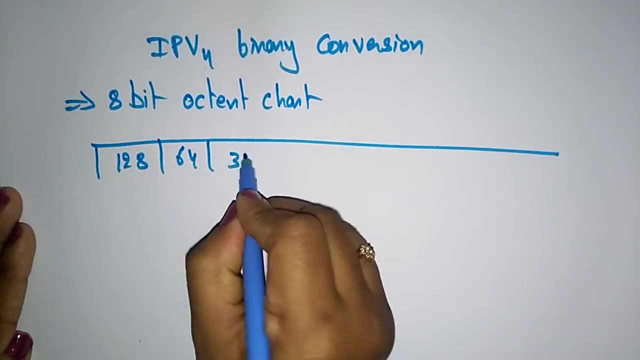 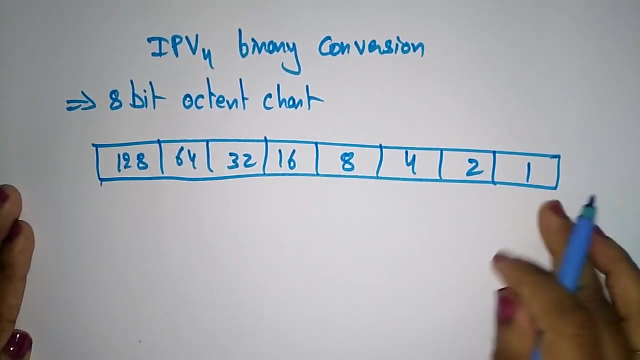 8-bit octant chart. So this consisting of 128-bit, 64,, 32,, 16,, 8,, 4,, 2, 1.. So this is a chart: 1,, 2,, 4,, 8,, 16,, 32,, 64,, 128.. 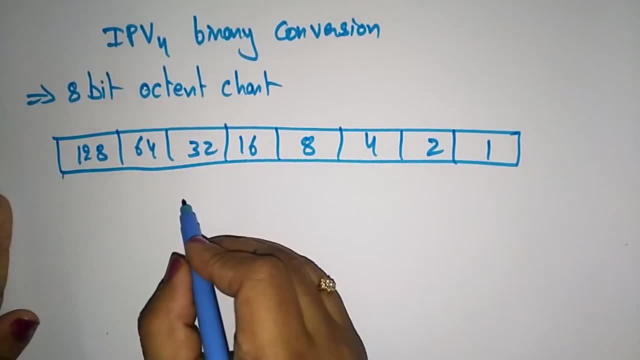 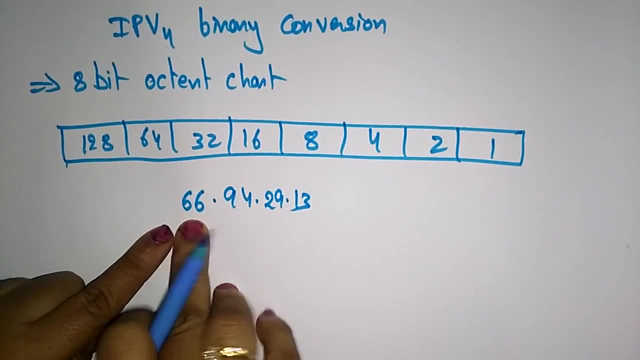 Okay, So Let me take the first, our decimal number 66.94.29.13.. So the first. let's take the first octant: How I can convert this into binary numbers. Okay, So how can I convert this into binary numbers? 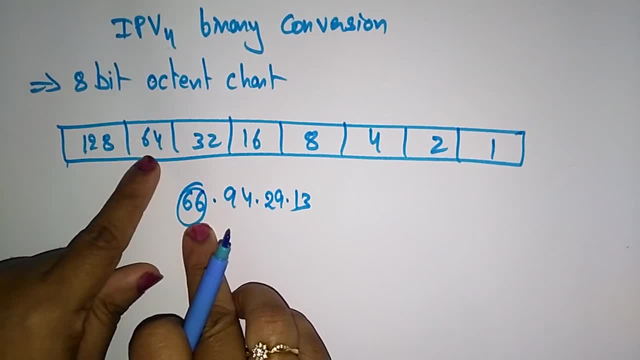 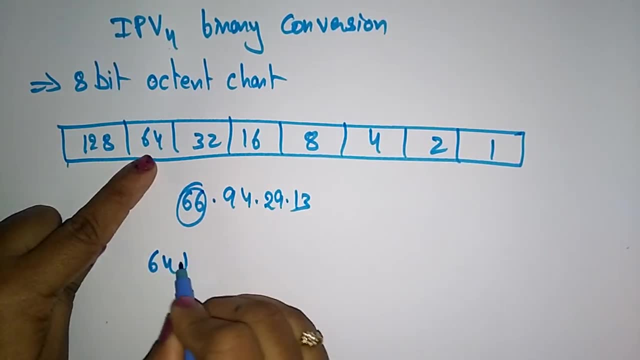 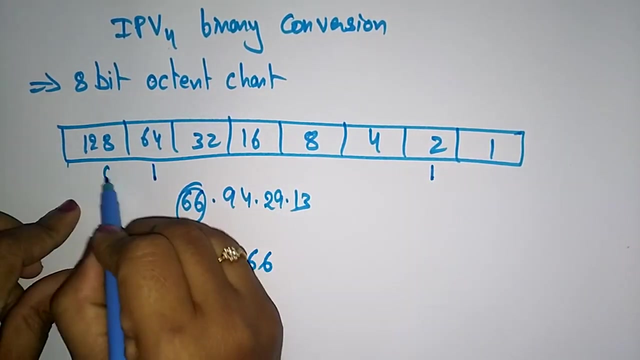 So let me take: 66 means 64 plus 2, you will get 66. Okay, Okay, 64 plus 2 is nothing, Right 66.. So just place 1 here and 1 in 2 and the remaining all 0s. 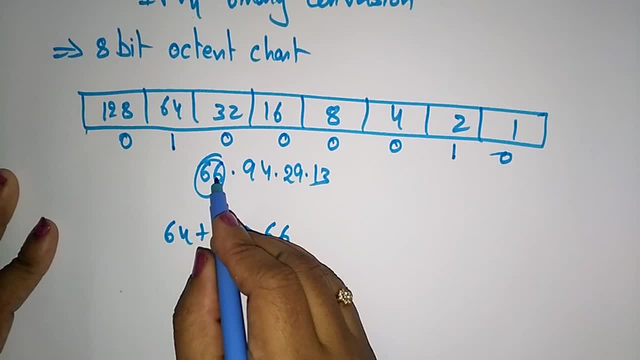 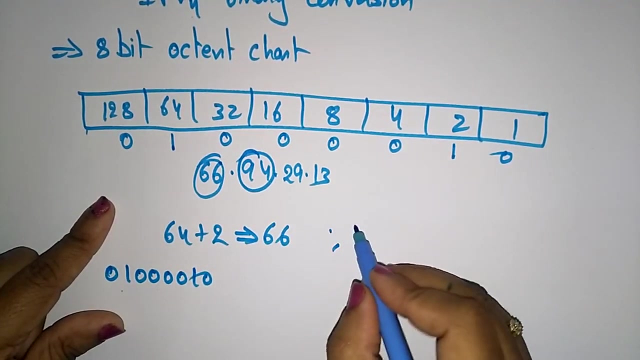 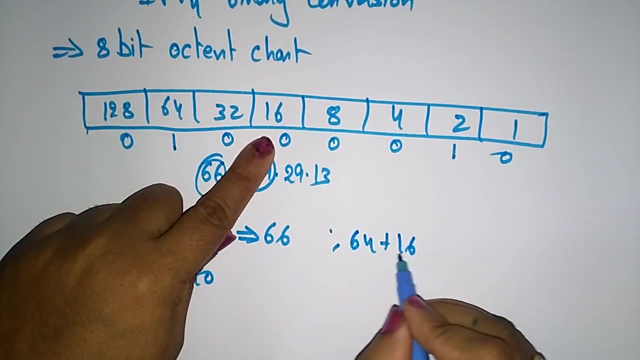 So that is the value of 66.. So the 66 decimal conversion to binary is 010000010.. So next is 94.. So 94 is a combination of: let's take 64 plus 16.. 64 plus 16, you will get total 10,, 80,. 80 plus 88 plus 4 plus 2, you will get 94.. 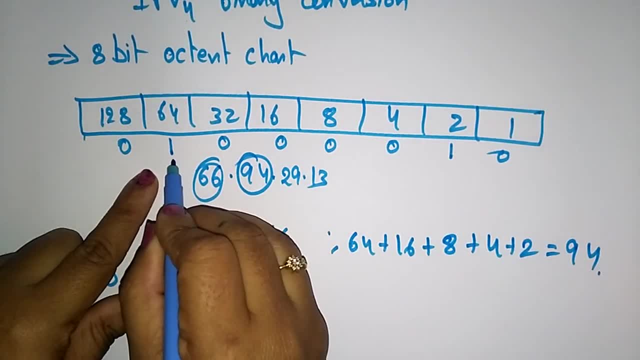 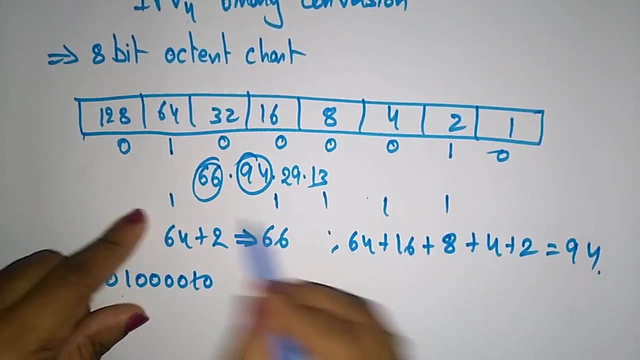 So in that places, just place 1 here, 64 is 1,, 16 is 1,, 8 is 1,, 4 is 1,, 2 is 1 and the remaining all are 0s. Okay, Then, what is our next? 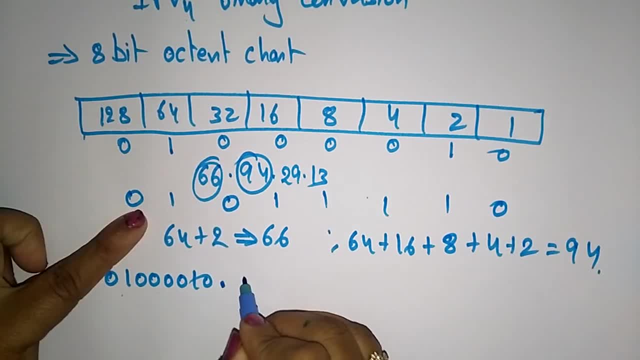 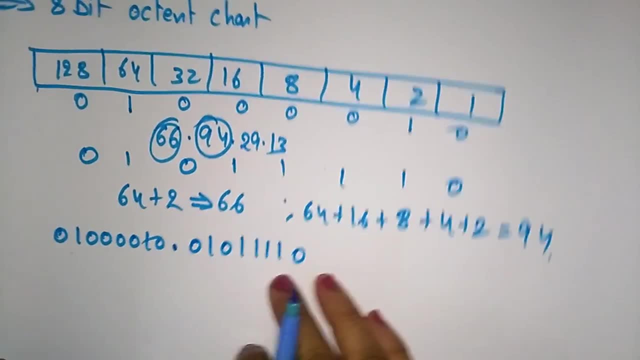 Next, 94,. 94 is a combination of 0,, 1,, 0, 1, 1,, 1, 1, 0.. So this is the way you will get the value. So, in the same way, you just convert all the decimal numbers into binary conversion.